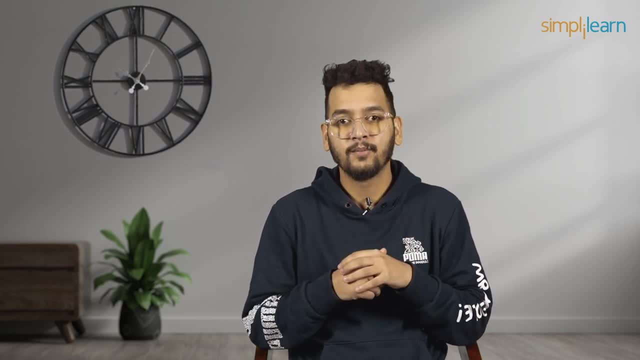 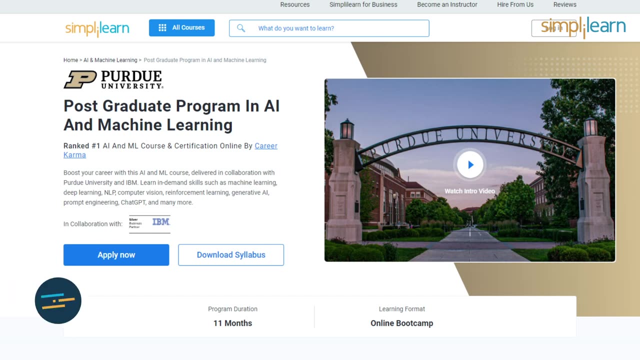 hands-on using the decision tree algorithm. Just a quick info for you: Decision tree is, after all, an algorithm that is based on AI and machine learning. A professional who wants to switch careers with AI and ML by learning from their expert? Then try giving SimpliLens. 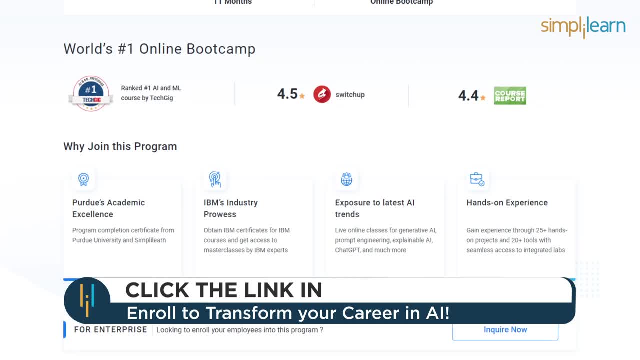 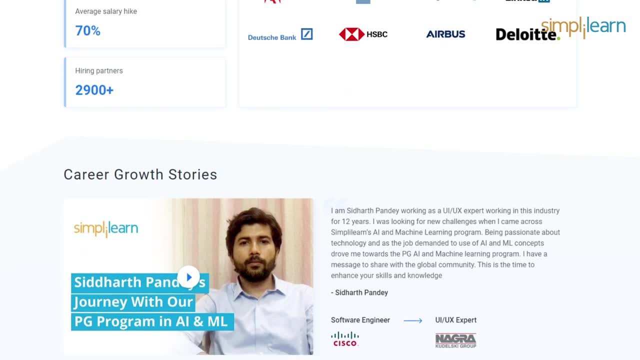 postgraduate program in AI and machine learning from Purdue University, in collaboration with IBM. In this AI and ML course, learn in-demand skills such as machine learning, deep learning, NLP, computer vision, reinforcement learning, generative AI, prompt engineering, chat, GPT and many more. 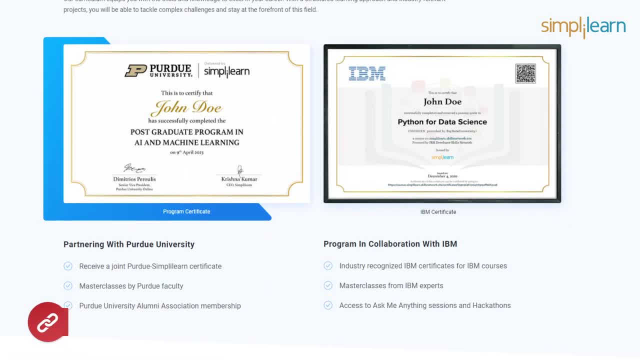 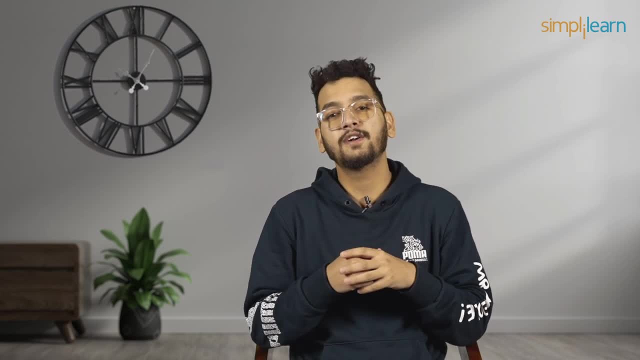 The link in the description box should navigate to the homepage, where you can find a complete overview of the program being offered. So take action, upskill and get ahead. So, without any further ado, let's get started. So what is a decision tree? A decision tree. 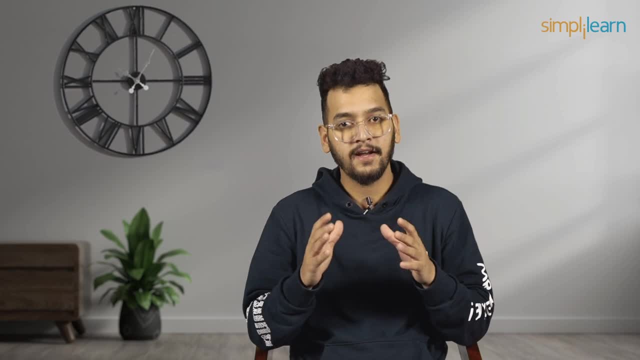 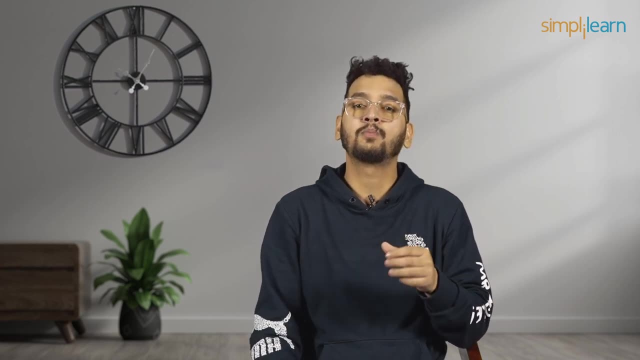 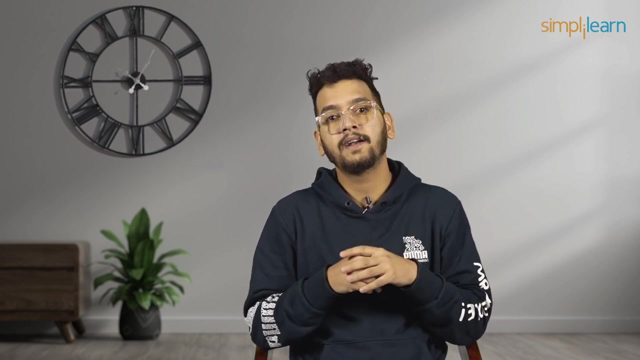 employed in supervised learning is a tree-like structure designed to forecast the outcome of a target variable In supervised learning, which relies on labeled data containing known output variables, predictions are made through regression and classification algorithms. These algorithms serve as guides in training a model with a 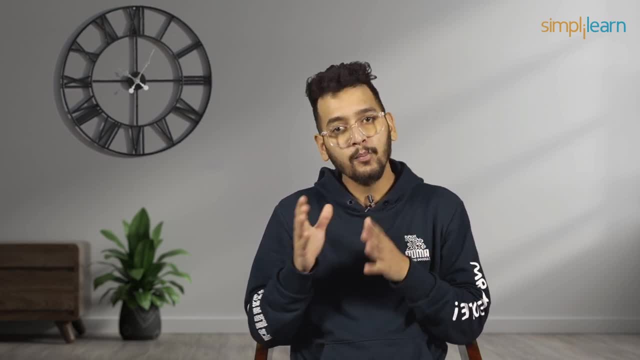 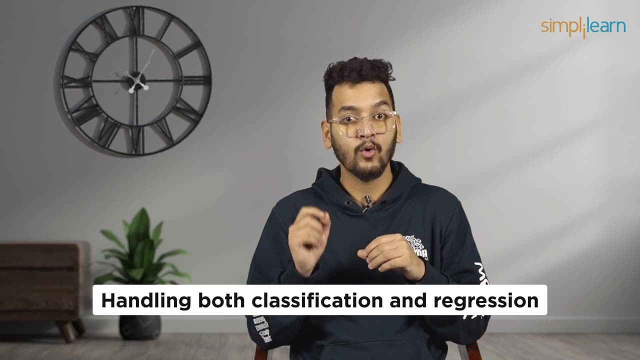 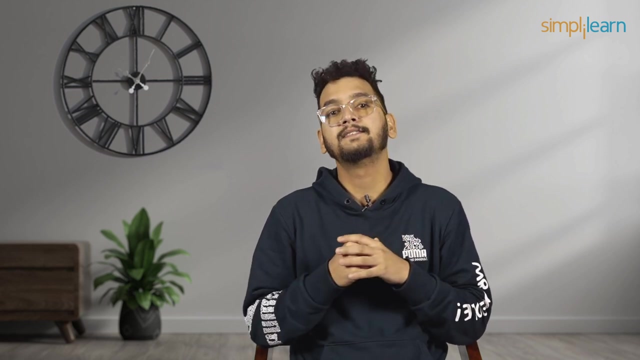 predetermined output variable. By grasping uncomplicated decision rules based on diverse data features, the model learns. Python's decision tree proves versatile, handling both classification and regression challenges, often finding applications in assessing probabilities. So, moving forward, let's see the advantages of decision trees. 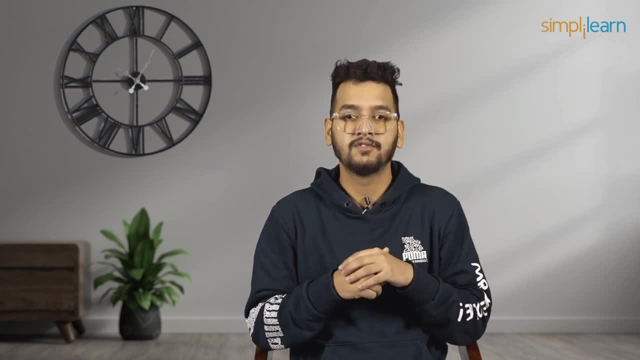 Decision trees are simple to understand, interpret and visualize. The second one is they can effectively handle both numerical and categorical data. The third one is they can determine the worst, best and expected values for several scenarios. The last one is they perform well, even if the actual model violates any assumptions. So, moving forward, we will discuss some decision. 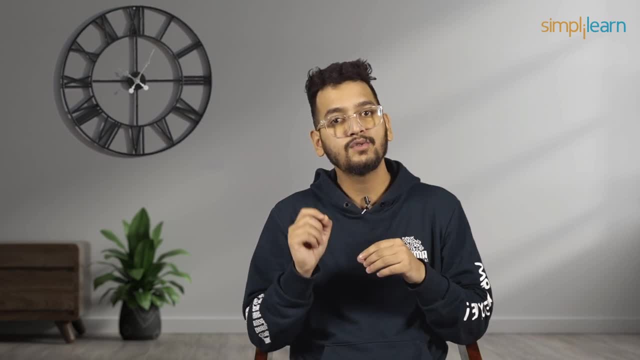 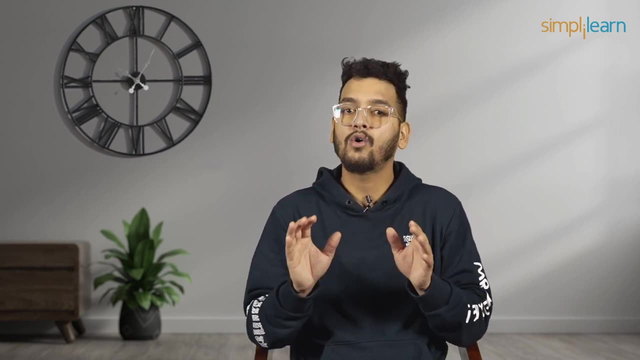 tree applications. So the first one is a decision tree is a tree-like structure designed to determine whether an application is likely to default on a loan. The second one is it can be used to determine the odds of an individual developing a specific disease. The third one is 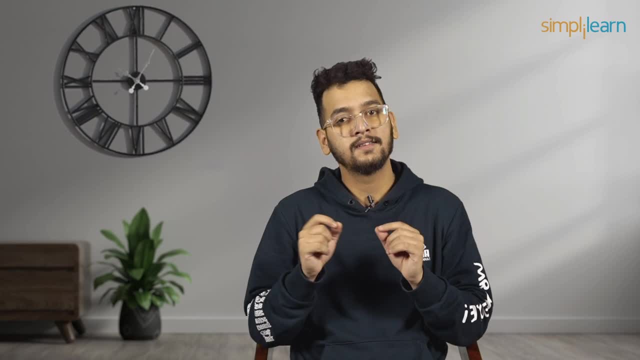 it can help e-commerce companies in predicting whether a consumer is likely to purchase a specific product or not. The fourth one is decision tree can also be used to find customer churn rates. So, moving forward, we will see some important terms used in decision trees. 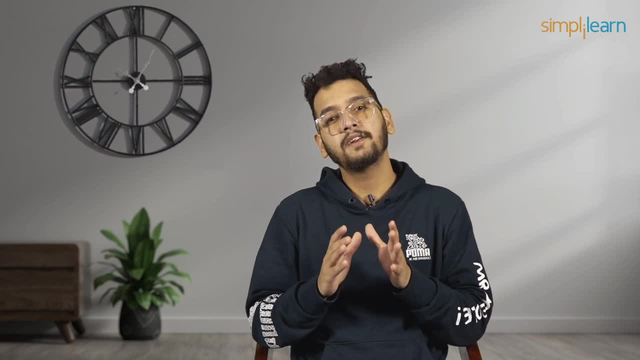 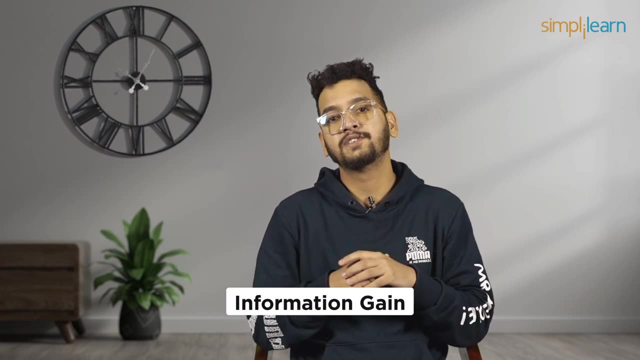 So the first one is entropy. Entropy is the measure of uncertainty or randomness in a data set. Entropy handles how a decision tree splits the data. The second one is information gain. The information gain measures the decrease in entropy after the data set is. 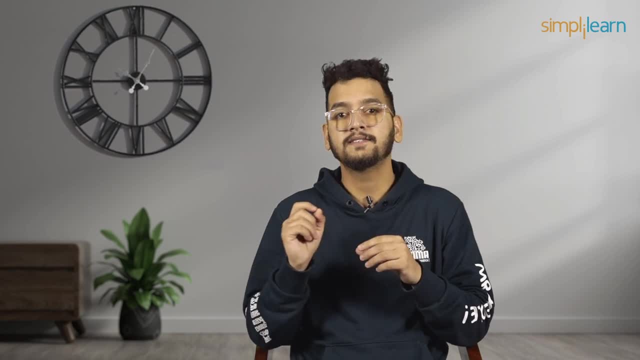 split. The third one is Gini index. The Gini index is used to determine the correct variable for splitting nodes. It measures how often a randomly chosen variable would be incorrectly identified. The fourth one is root node. The root node is always the top node of a decision tree. 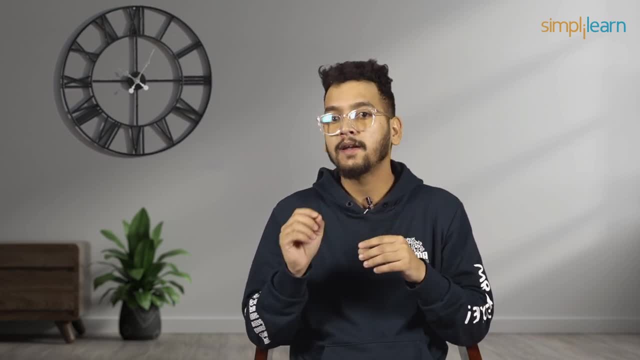 It represents the entire data set. The third one is a decision tree. It measures how often a decision population or data sample, and it can be further divided into different data sets. the fifth one is decision node. decision nodes are the sub node that can be split into different sub nodes. 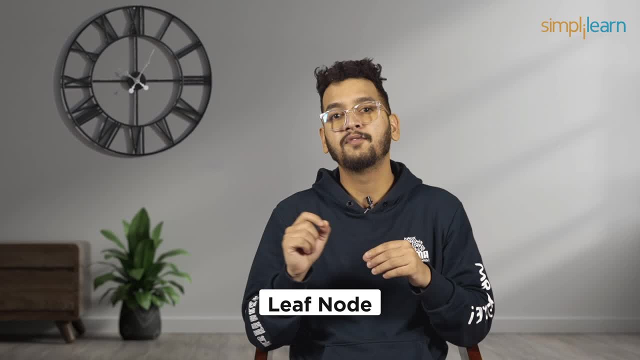 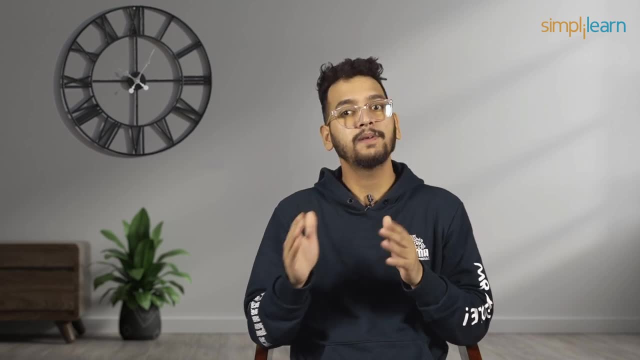 they contain at least two branches. the sixth one is leaf node. a leaf node in a decision tree carries the final result. so these nodes, which are also known as terminal nodes, cannot be split any further. so let's move forward to the demo part. so first we will rename this jupiter notebook. 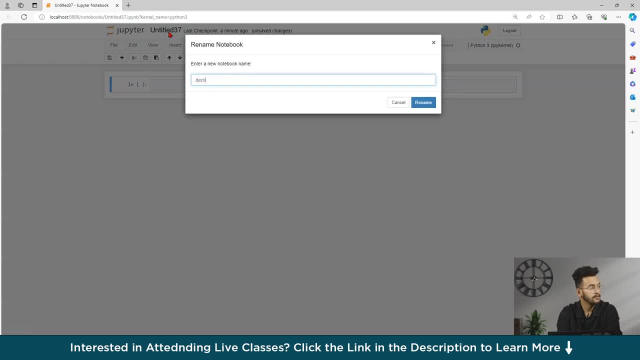 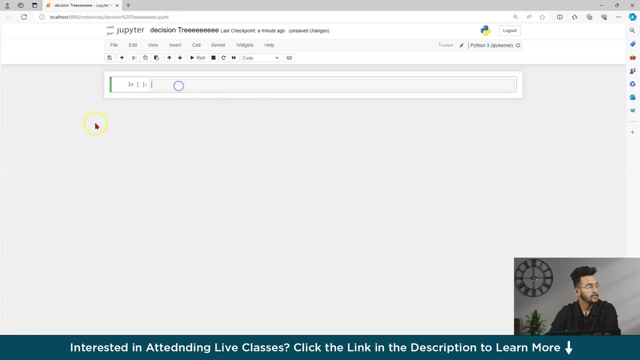 uh, like this season, this is entry right, okay, okay. so first we will import some major libraries like numpy, pandas, matplotlib, sklearn, seaborn. so first we will import, import pandas as pd- right, it is pandas pd. then i will import numpy numpy as np, then i will import matplotlib, dot pyplot as plt. 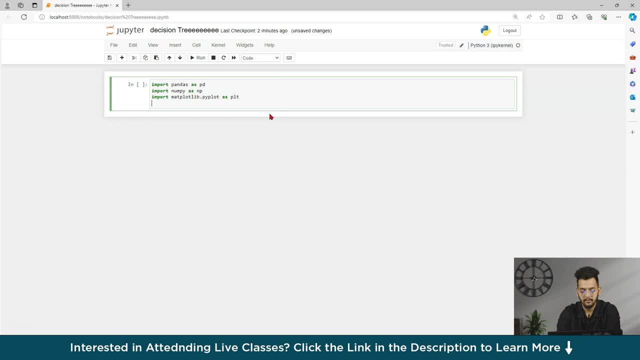 then we will import sklearn and then we will import metrics on them. so, from sklearn, import metrics. right, then we will import seaborn- seaborn as sns- from sklearn dot data sets. okay, i will import load iris, so i will import the iris data set. that's flower one. then, moving forward, we will import some model selection: sklearn dot model selection import train. 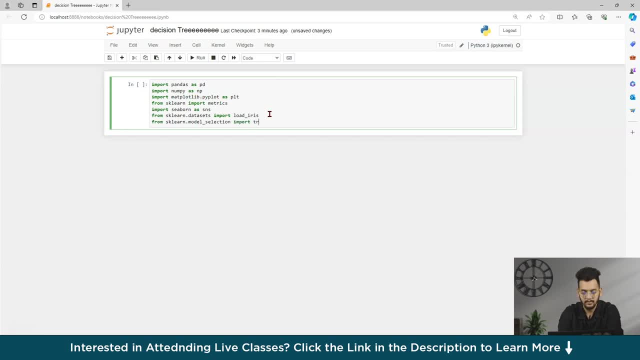 test: split model selection. import train test: split model selection. import train test. split model selection. import tree: we will make decision tree like tree shape structure. okay, so let me done is: yes, everything is fine. okay, it's still loading. yeah, so, everything is fine. so moving forward. we will import data set. 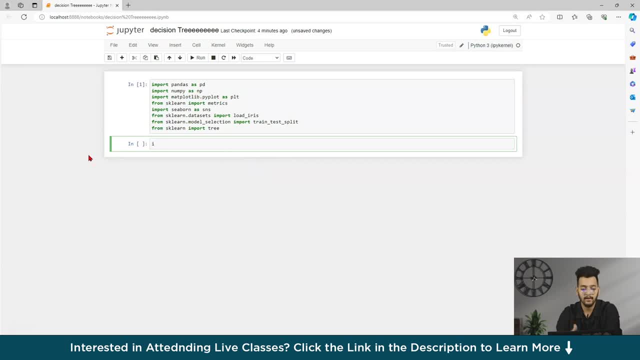 okay, so everything is fine. so, moving forward, we will import data set. moving forward, we will import data set set. or you can say the load data set below data that iris equals to load iris, right, yes, it's working fine. then data goes to PD dot data frame and data equals to iris dot data. okay, then comma columns. 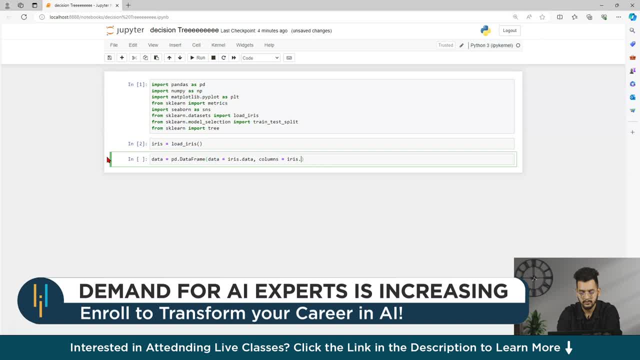 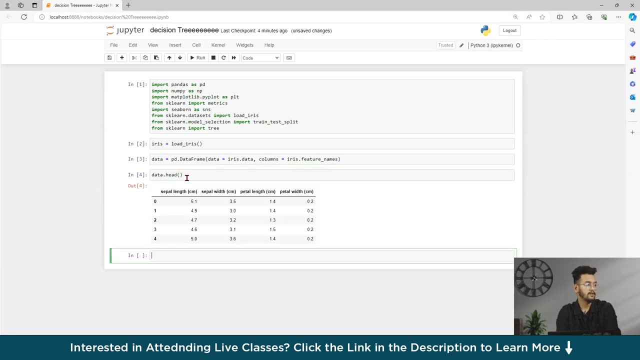 equals to iris dot feature names. okay, and I will run it if I will check data dot. okay, and I will run it if I will check data dot. okay, and I will run it. if I will check data dot head what it will show: see, you can see the data set: sepal length, sepal width. 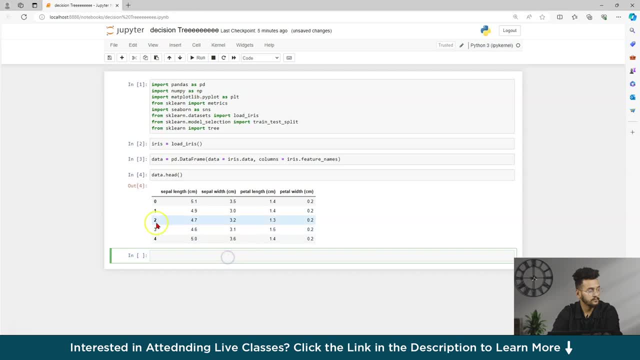 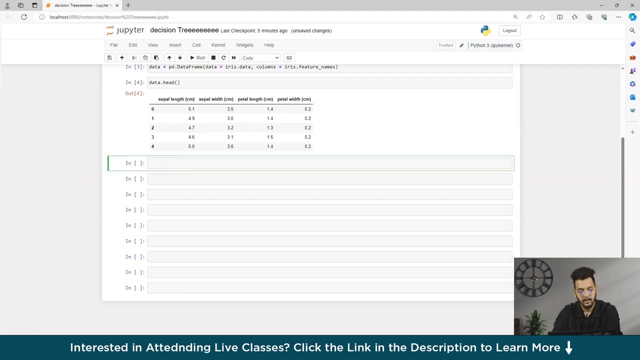 petal length, petal width. okay, yes, first give me yes. so let's make species as a target variable. ok, suppose I will write her data: species goes through. r is dot target. then I will write a target. it cost you and be dot unique and I'll. 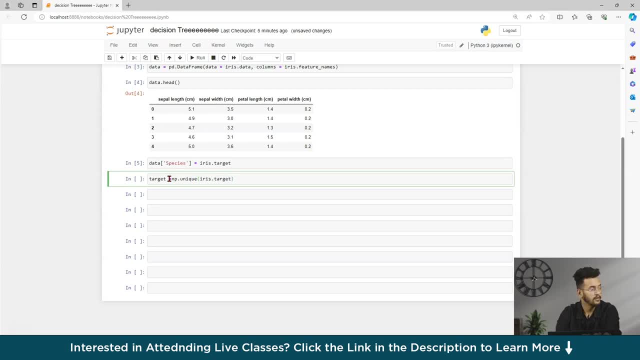 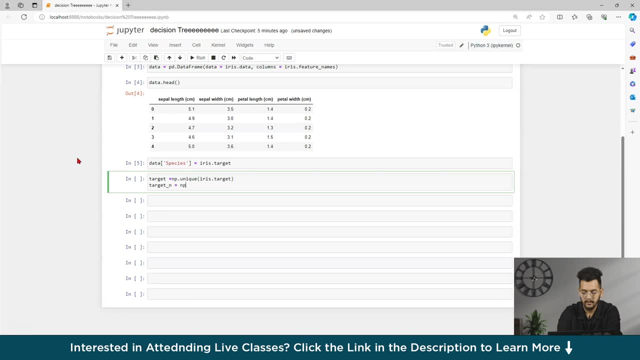 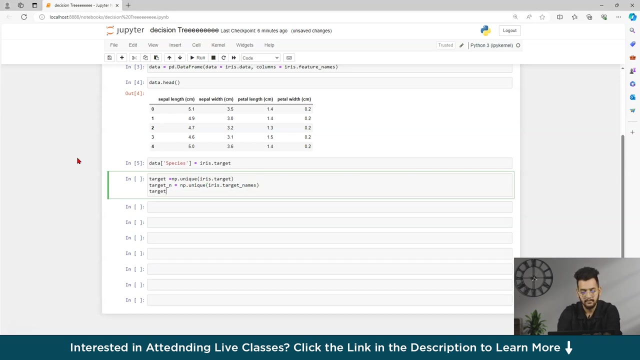 relate administrative. OK, say that, very simple rounding programming: target variable. are you suppose the target variable is represented as the palliative? I will write a right enter target target. I just dot target. okay, then I will write: target and variable equals to NP dot unique, then iris dot target names. okay, then target dictionary. 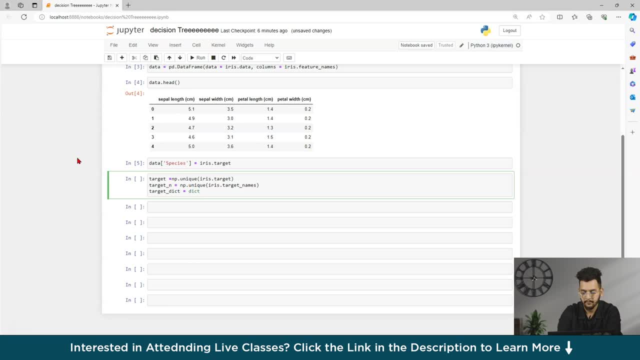 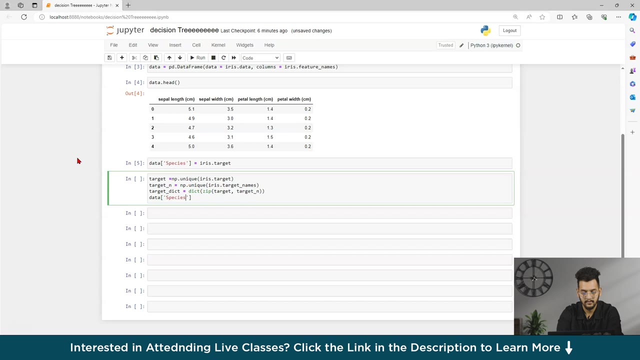 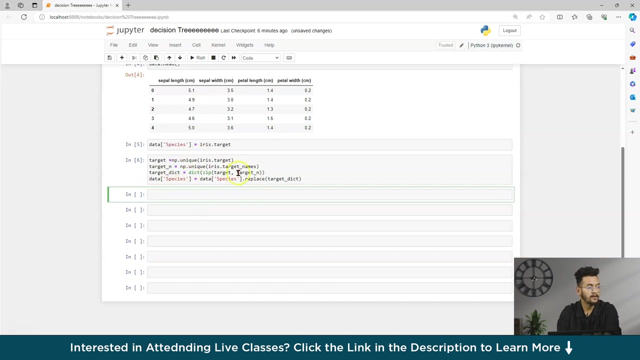 equals to dictionary in zip file, then comma target, comma target and underscore n. right, then, moving forward, I will write: data species goes to data species. dot replace target dictionary. right, we run it. okay, it's working fine. so we set target as a species. okay, then now what we will do. we will make X and Y column. okay for the. 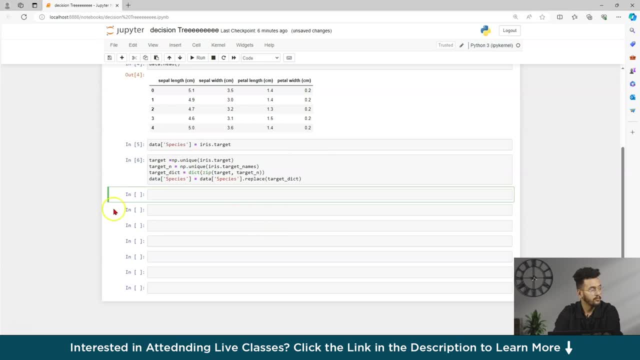 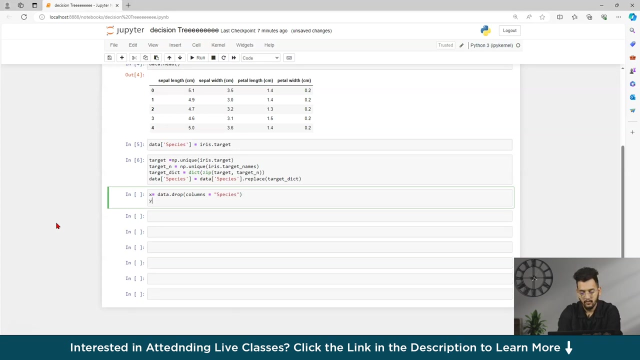 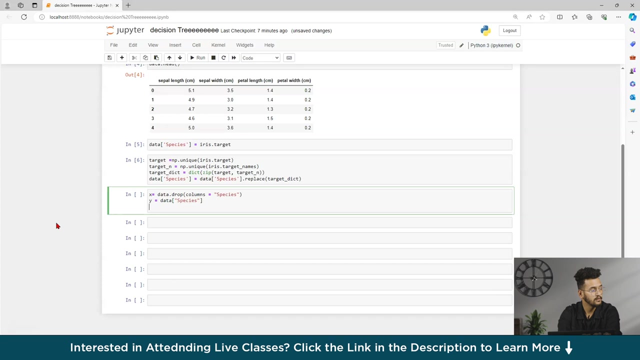 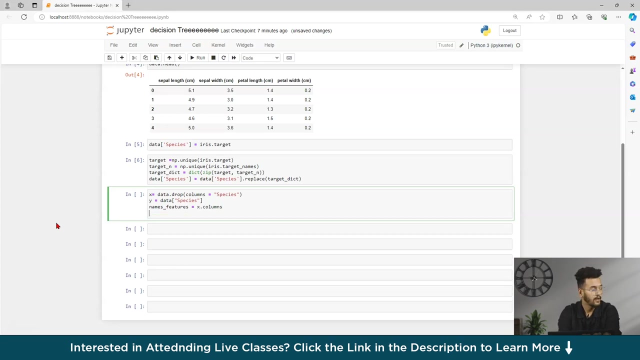 train and test split. so I will write here: X equals to data dot drop columns, right equals to species. then Y goes to data, again species, right. then names underscore features equals to X dot columns. we are assigning names features to X column and here I will write target labels. 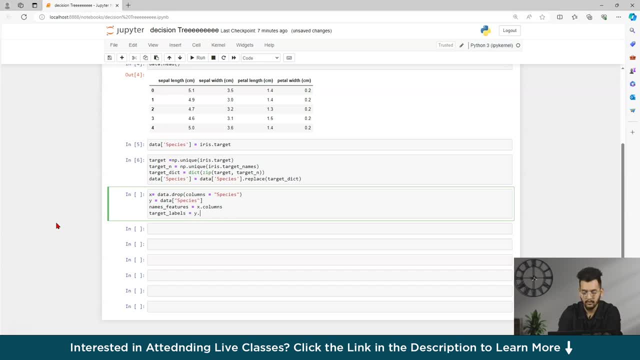 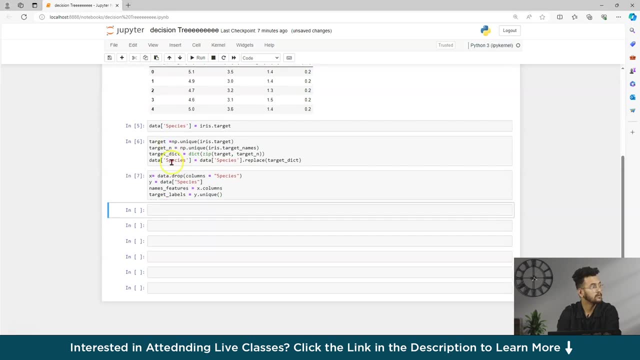 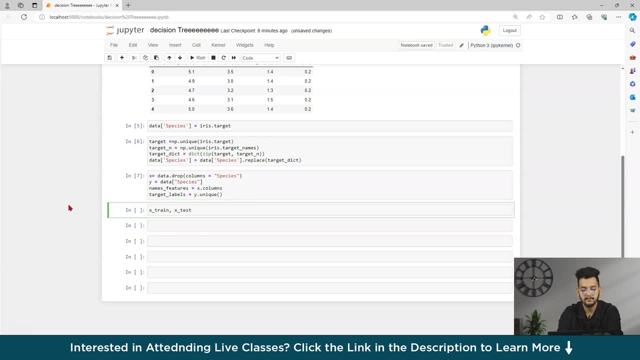 and the test okay. so X: underscore train comma X underscore test comma Y underscore train comma Y. underscore train comma Y: underscore test equals to train test. split comma X: underscore test comma Y. underscore train comma Y: underscore test equals to train test. split X, comma Y. comma X: underscore test comma Y underscore train comma Y: underscore test equals to train test. split X, comma Y. 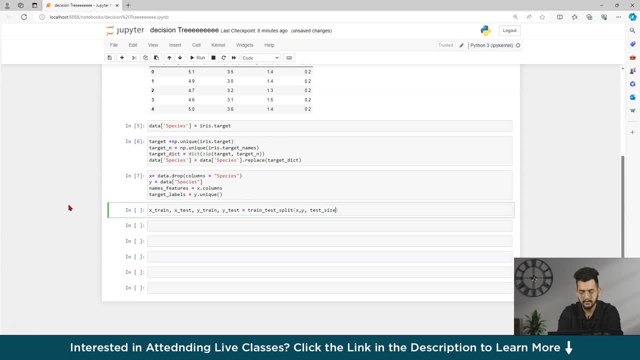 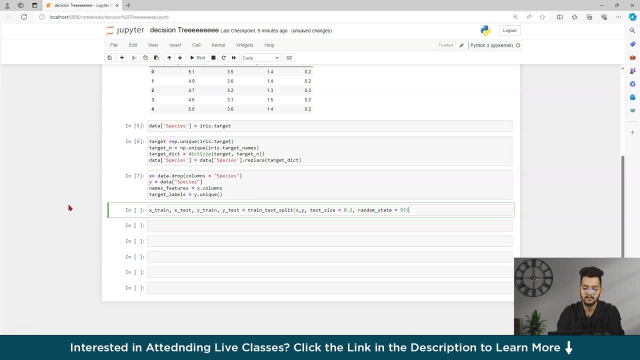 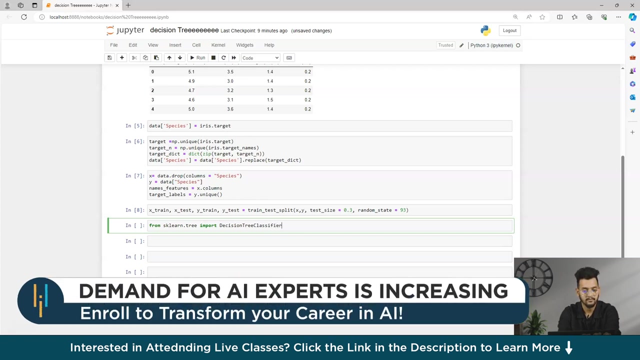 percent means training data. the 30 percent is remaining is the testing data. okay, so i will run it right. so here i will write from sk: learn dot. pre import: this season decision tree classifier. okay, then here i will write dtc, because i can't write this entry classifier again and again. 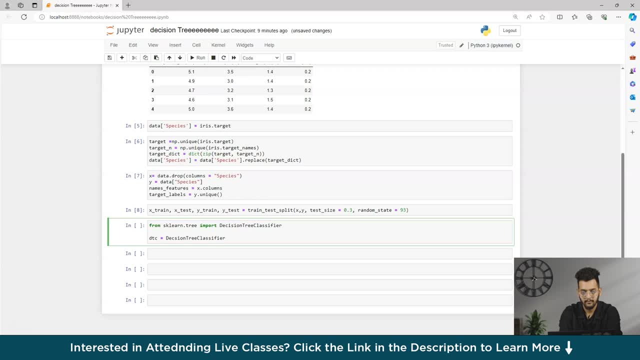 decision tree classifier. max depth equals to three comma. random state equals to 93.. okay, dtc dot fit. okay, 93, no, it's comma random state is 93 equals to 93? right then, dtc dot fit x train. comma y train. okay then plt dot figure. 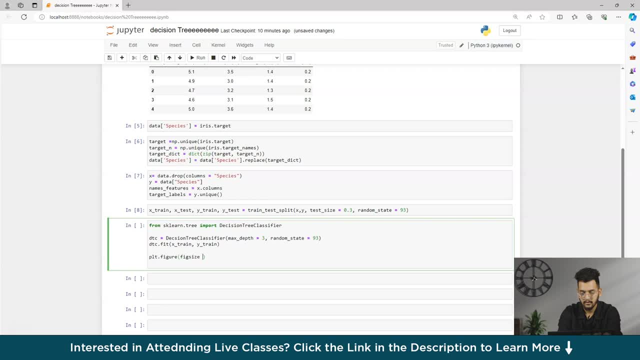 then figure size equals to 30 comma. 10 comma. face color will be a phase color equal to b. then i will add tree equals to treeplot, underscore tree. then dtc is entry classifier: comma features, name features: yeah, features name. comma features. comma class names equals to target labels. comma rounded was true. true then, 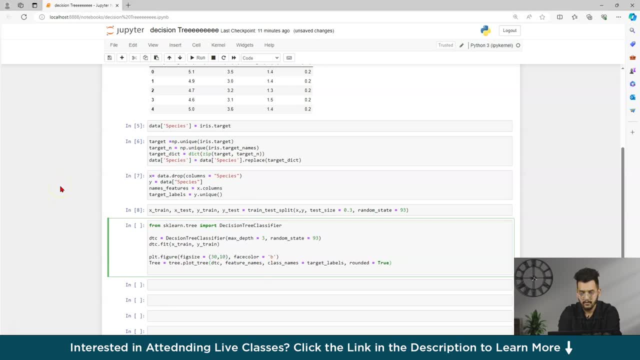 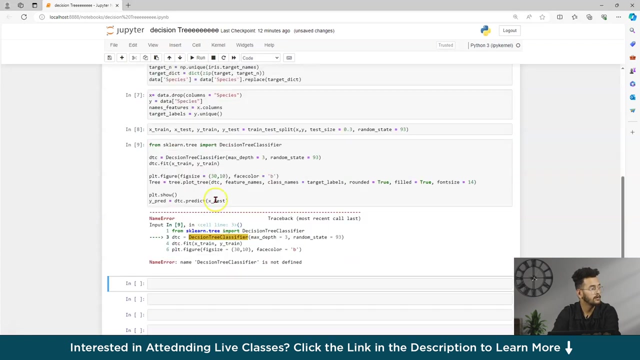 I will write comma filled with two values. comma font size will be 14. okay, yes, so now I will write here: PLT dot show. okay, then Y prediction equals to DTC dot predict X test. okay, this is entry. classifier is not defined. maybe some spelling mistake is there. 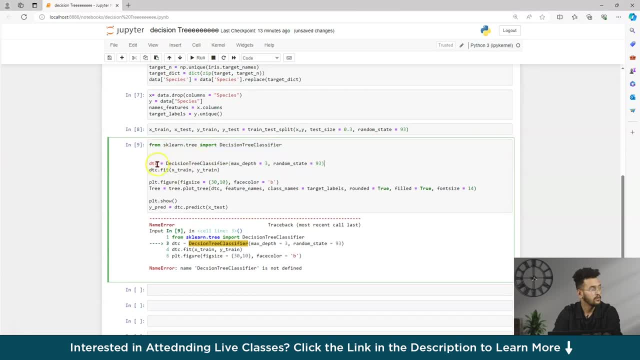 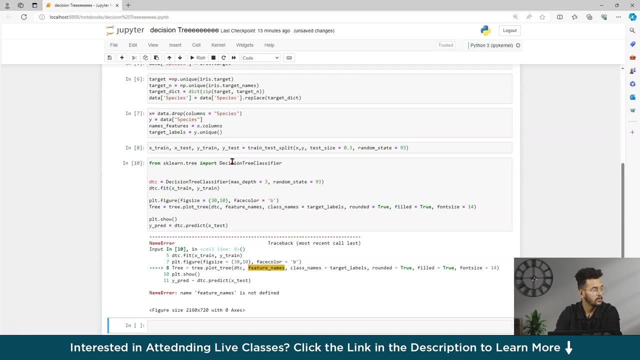 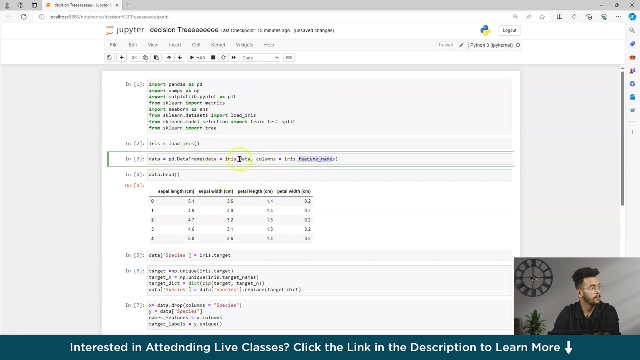 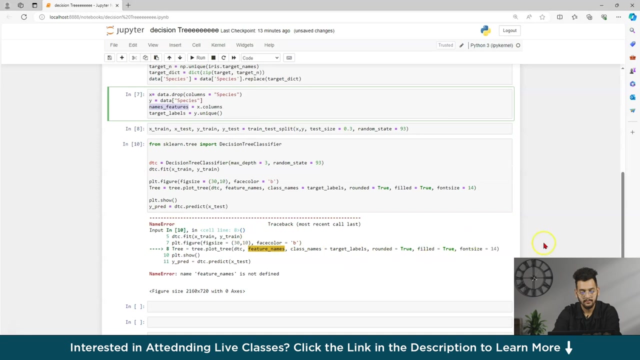 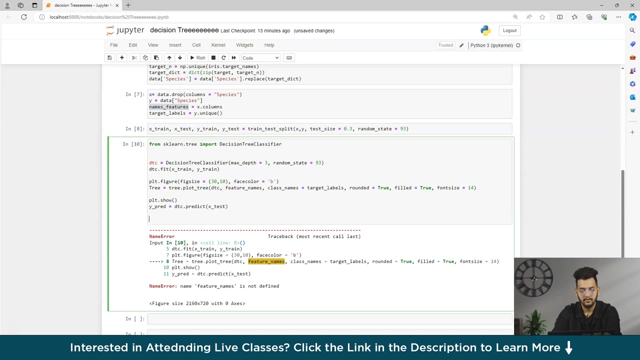 okay, okay, let me check now. okay, feature names is not defined, just name bigger's name. okay, this name is underscore features. So what I will do? I will write first full code, then I will show you the both graphs. so I will write here: confusion: underscore matrix equals to matrix matrix dot. confusion. 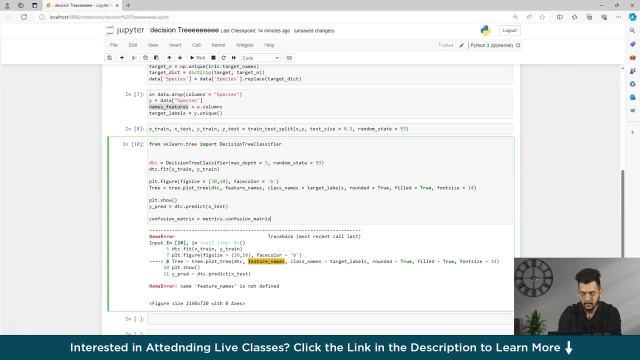 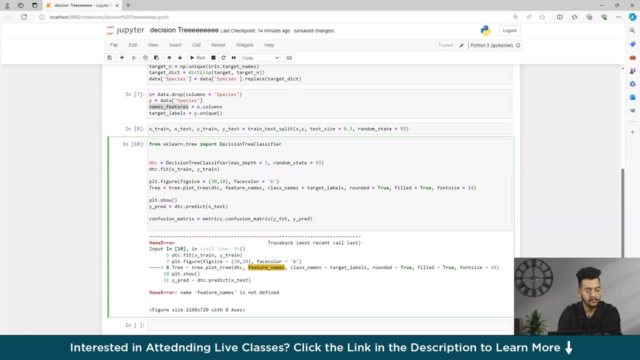 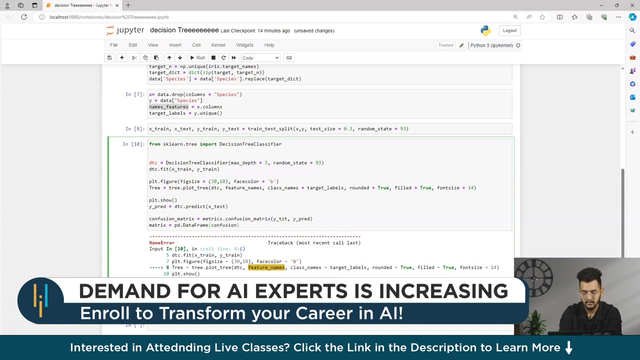 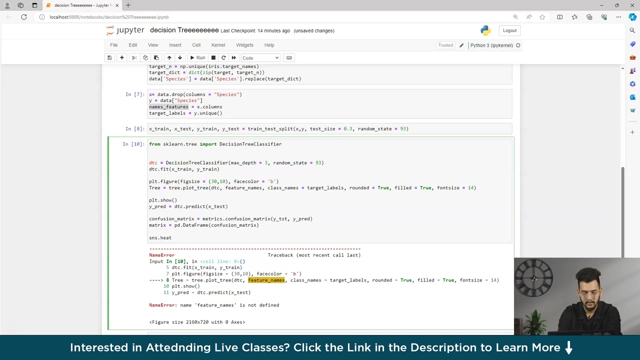 matrix: Okay, Then Y test comma, Y prediction: okay, then matrix equals to PD dot data frame, then confusion matrix: Okay, we will create one confusion matrix graph heat map. Okay, So I will write sns dot heat map: matrix comma not equals to true comma, fmt equals to g comma. 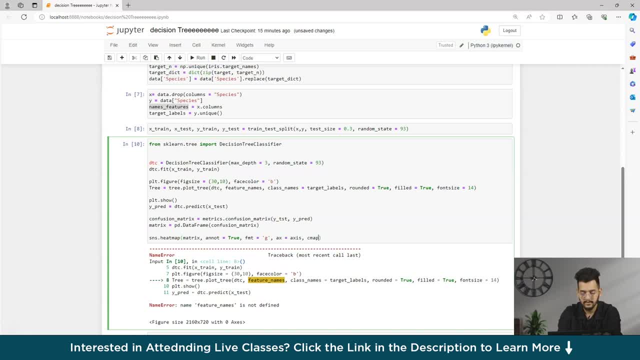 axis equals to axis comma. cmap, sitemap equals to true. Okay, Okay, So I will write here magma, then axis dot. set. title is confusion matrix. Okay, Then we will set the x label, x tick label, y label, y tick label. 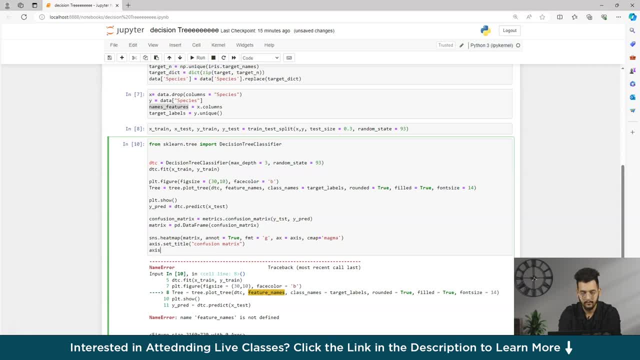 Okay, Then I will write here: So: axis dot set x label predicted value: comma font size equals to 10, then axis dot set x ticks label labels. okay, plus target labels. then access dot set why tick labels, and list will become. then target labels will show. then I need. 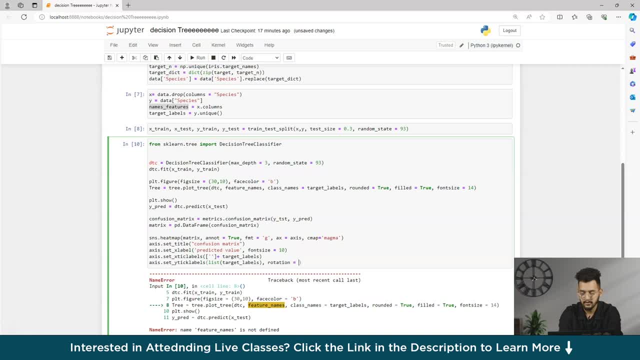 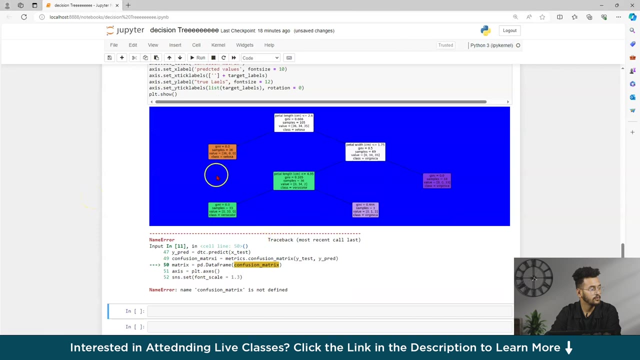 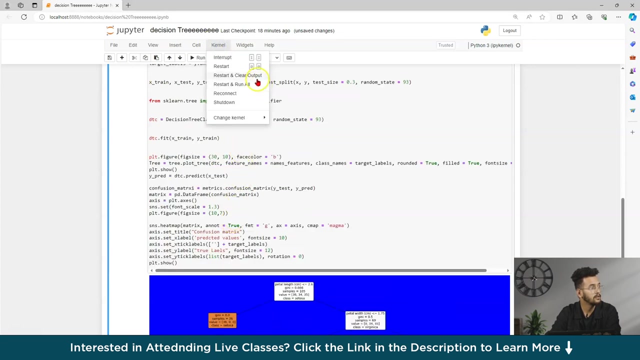 one rotation of 0 and it goes to 0, then I will write PLT dot show. okay, so let me run it so as you can see, the decision tree is here, but there is confusion with confusion matrix. okay, first I will start and clear all outputs. I will do and let 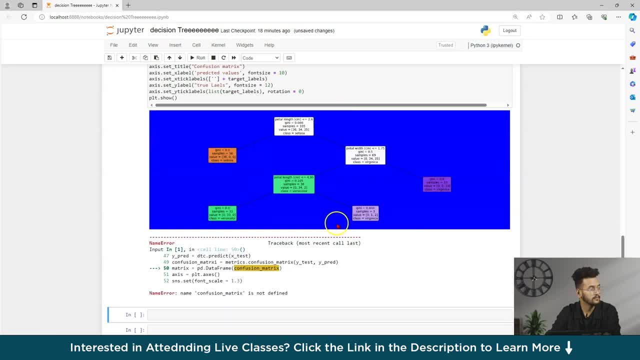 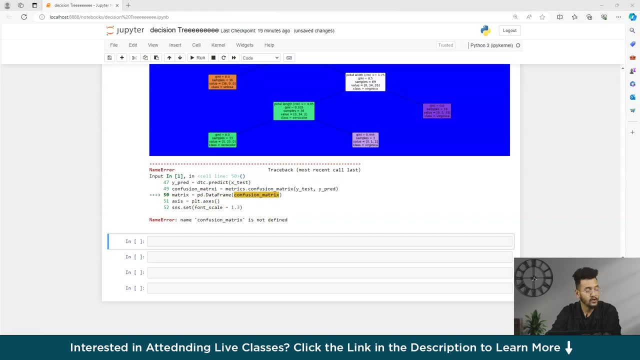 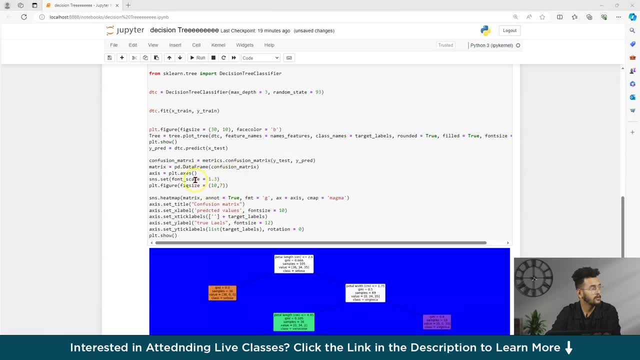 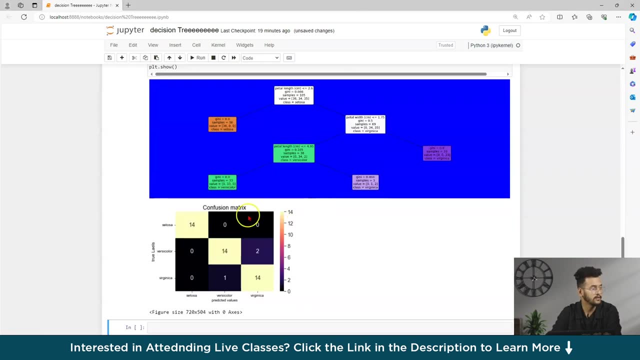 confusion: matrix is not defined. okay, it's matrix, now it will come. yes. so, as it's matrix, now it will come. yes. so, as it's matrix, now it will come yes. so, as you can see confusion, matrix is here and you can see confusion, matrix is here and 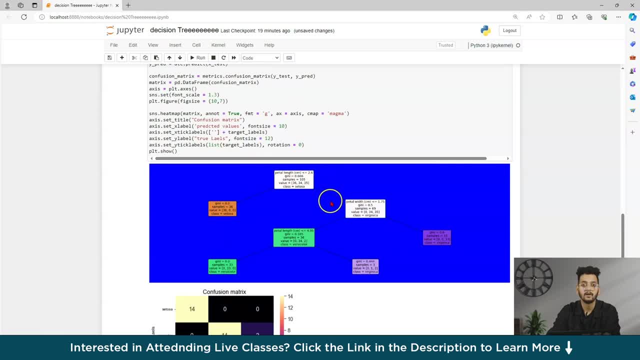 you can see confusion. matrix is here and the decision tree. this is how you can the decision tree. this is how you can the decision tree. this is how you can make the recent tree. we already discussed. make the recent tree. we already discussed. make the recent tree. we already discussed this word: Guinea, right the same. 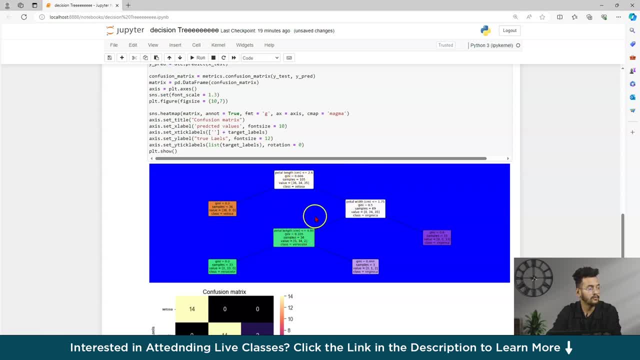 this word Guinea, right the same. this word Guinea, right the same. pulse values: so these petal and petal pulse values. so these petal and petal pulse values, so these petal and petal width are from the data set, got it. and width are from the data set, got it. and